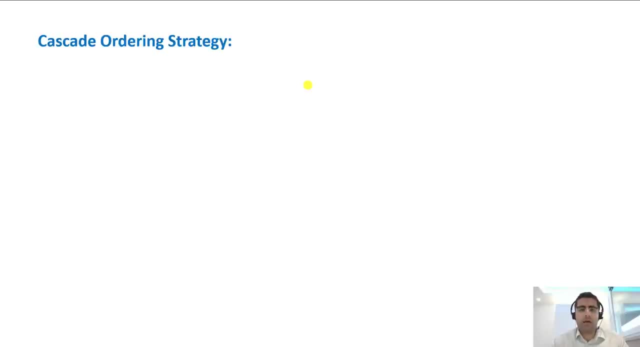 And in the third section I will show you the results and test this strategy by using strategy tester And we can see the performance of this strategy. If this is your first time watching our channel, I would really appreciate to hit subscribe button. In this channel we focus on different strategies in Forex, Crypto and Stocks markets. 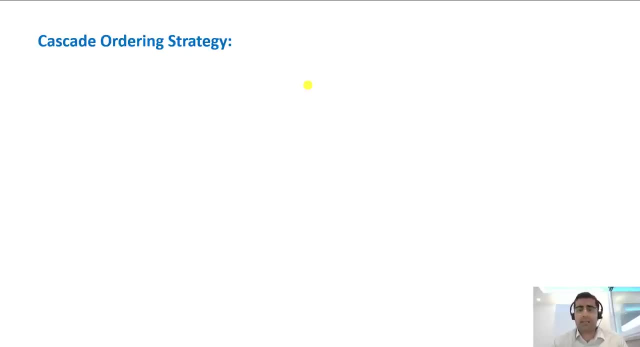 And specifically on making transactions, Making an algorithm for them and using algorithmic trading in our daily tradings. If you have any suggestion for upcoming videos and you want me to make a video regarding them, I would really appreciate to leave me a comment. 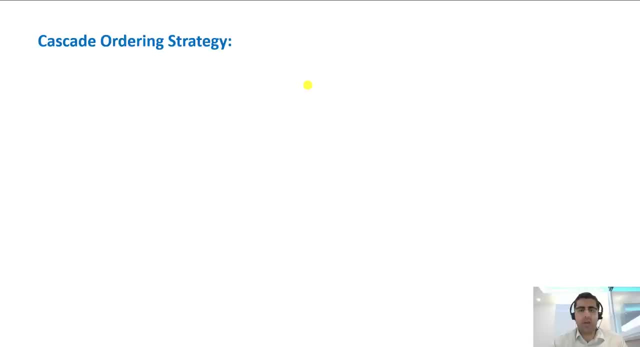 I will read them and consider them for upcoming videos. I hope you enjoy this video and stay with me to the end. Normally, when we open an order based on any strategy and we enter into the market, we have a stop loss, for example, 10 points or pips lower than the entry point. 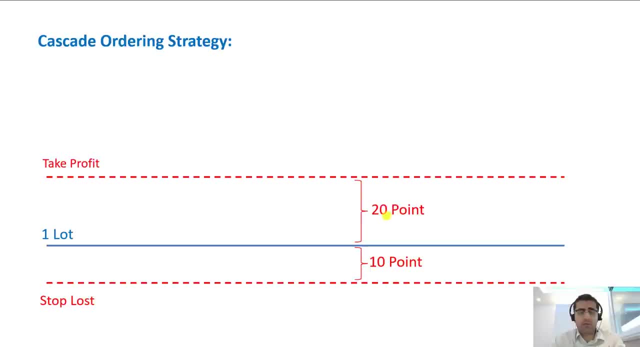 And if the risk to reward is 2, we put the take profit 20 pips or points higher than the entry point, And whenever the price goes high and it goes in our favor and hit the take profit, we close the open order. And if it goes down and hit the stop loss, we close the order with losing money. But with this strategy, instead of closing the order when we hit the take profit, we open a new order exactly with the same lot size and transfer the stop loss to 5 points lower than the new open orders. 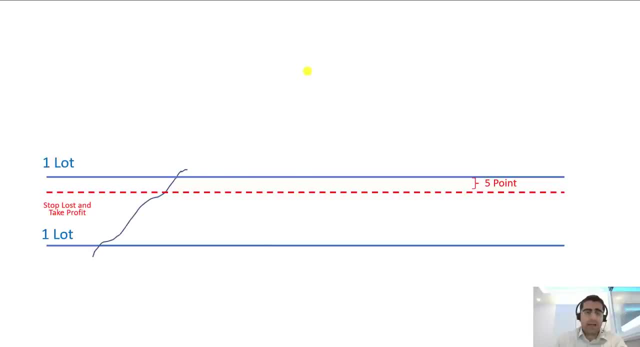 And we hope that the price goes higher and we make more money, Because in this case we have two open orders. But In this scenario is that the price does not goes in our favor and it goes back and hit this stop loss, which is, in this case, is stop loss for second open order and take profit for the first open order. 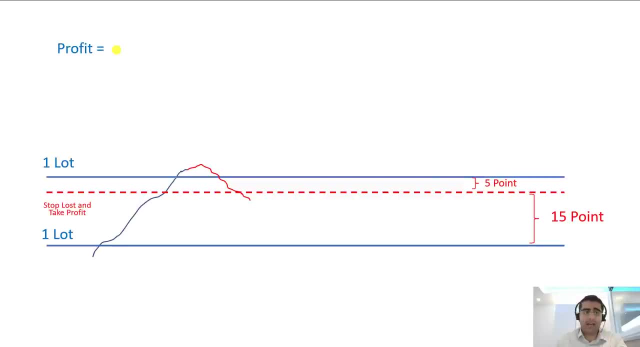 We calculate the profit that we have in this scenario, The profit would be one lot multiply 50 point. one lot for this order, which gained 15 points plus minus one lot multiply 5, for this open order, which it lost for 5 points, and the result would be 10 unit. 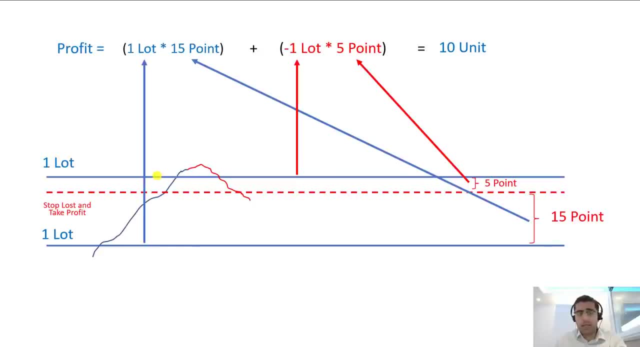 So if we didn't do that, then we would have gained 20 points, 20 units, and now we have gained 10 units. But we continue. We continue and see other scenarios. Imagine that price goes in our favor And 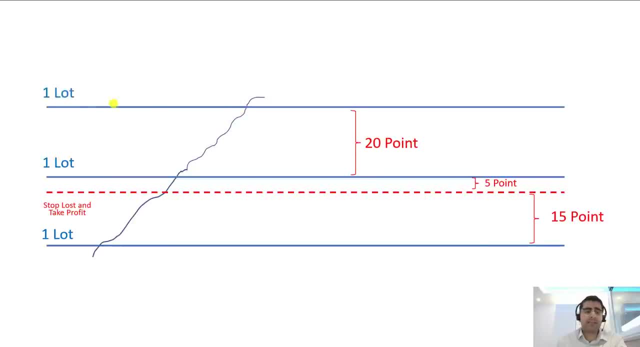 Increase by 20 points. In this case, again, instead of closing the order, we open a new order with exactly the same lot size and we transfer the stop loss to 5 points below the new order, And in this case then this line would be take profit for the first and the second order. 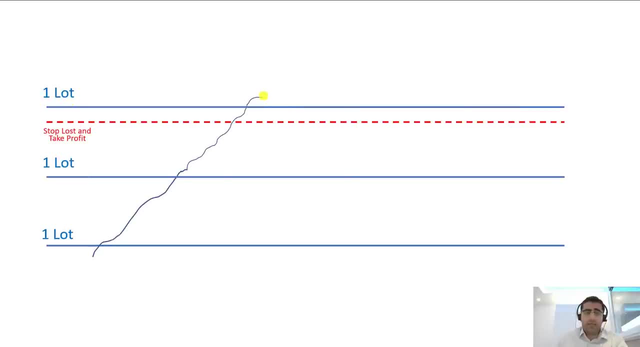 and stop loss for the third one, And we are hoping that the price goes even higher And we gain. we multiply actually our profit. But the first scenario is that the price doesn't do that and it goes back and hit this stop loss. 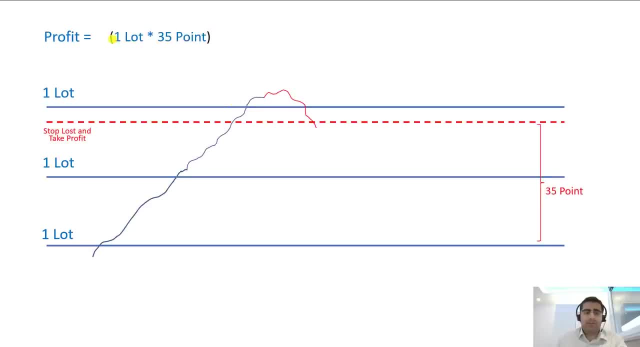 And we calculate our profit. The first profit that we have is one lot multiply 35 regarding the first order, plus one lot multiply 15 points regarding the second order, and plus minus one lot multiply 5 points regarding the third open order, which lost three, five points. 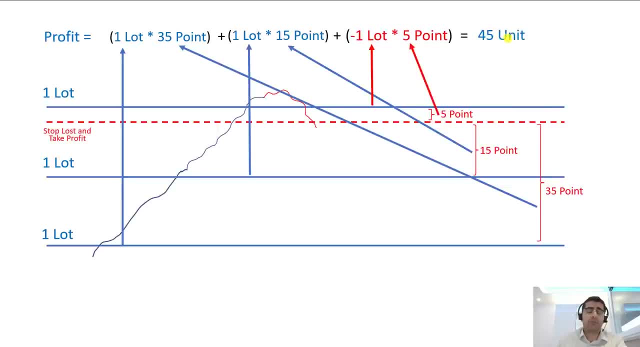 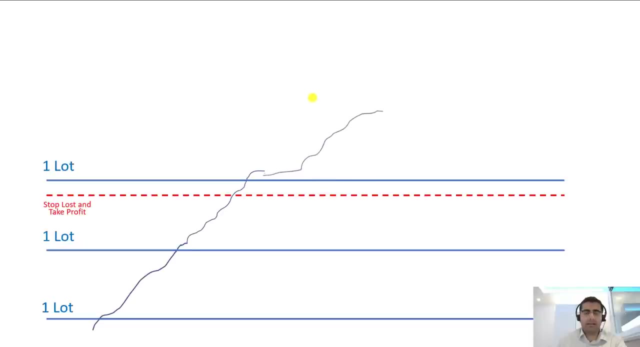 In this case the profit would be 45 units. See, It's increased very fast, But again we continue. We continue the scenarios. Now imagine that again price goes even higher And after 20 points we open again another order. 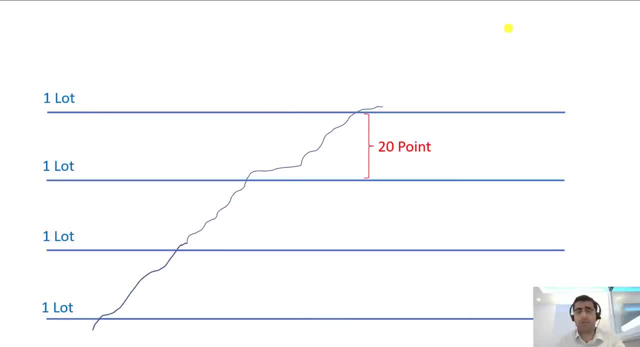 And we hope that price goes higher. So our profit would be multiply And we transfer the stop loss 5 points lower than below the first order, which is only the stop loss for this order, and take profit for the others. Again, we hope that the price goes higher. 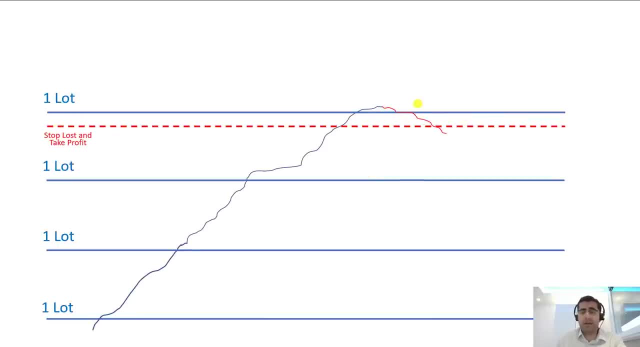 But in this case, the first scenario is that the price goes higher, goes down and hit the stop loss and we calculate the profit. The profit would be 1 lot multiply 55 regarding the first order: plus 1 lot multiply 35 point. plus 1 lot multiply 15 point. 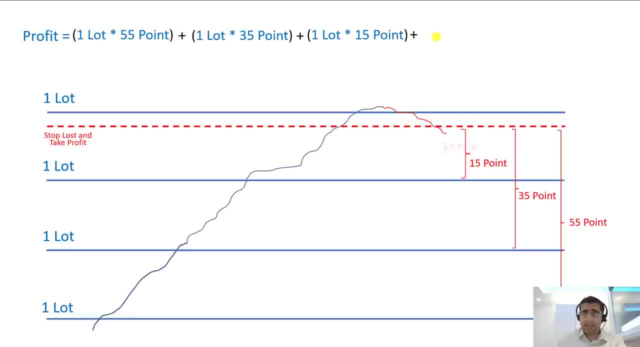 regarding the second and the third open order and plus minus 1 lot, multiply 5 unit regarding the last order, And then in this case we gain 100 unit. So imagine that only once per month we get to this point and we hit the fourth open orders. 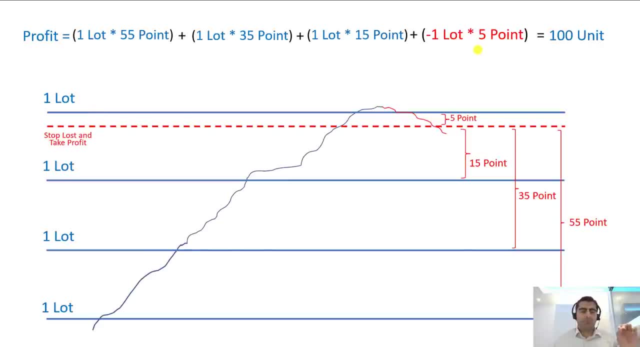 In this case, we need to be wrong in 10 other orders and we hit the stop loss for the next 10 orders to lose this profit, This money that we gained here. Statistically speaking, this way of closing the order is perfect actually. 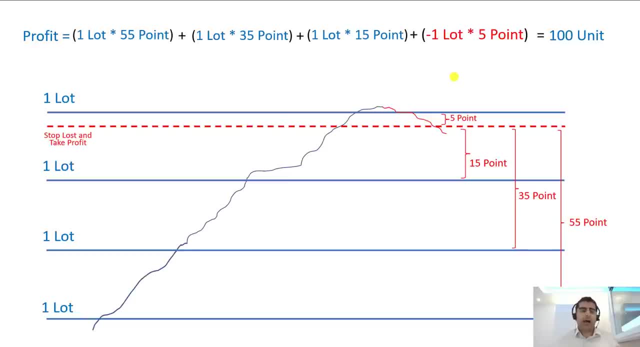 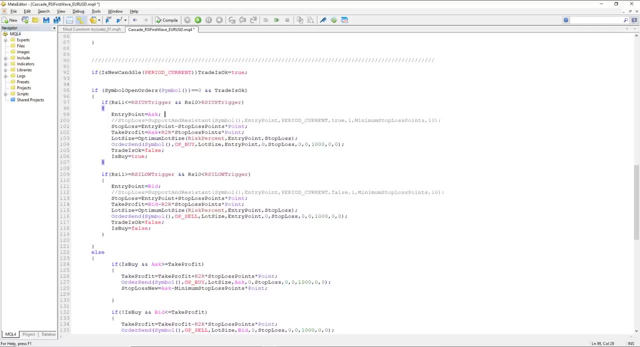 I have worked with that a lot. In the next section I will teach you how to program this strategy, and in the last section we will test this strategy by using strategy tester. Stay with me. So in this part of the video I will show you how I program. 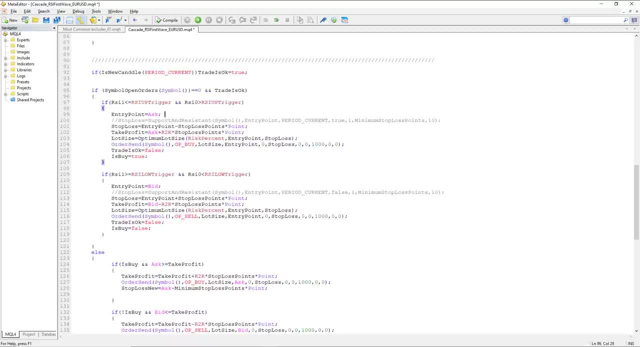 This strategy with MQL4 language. If you are not interested in the programming site programming section, I will suggest you to pass this video to the minute and the second that you can see here to see only the results of this strategy and its performance. 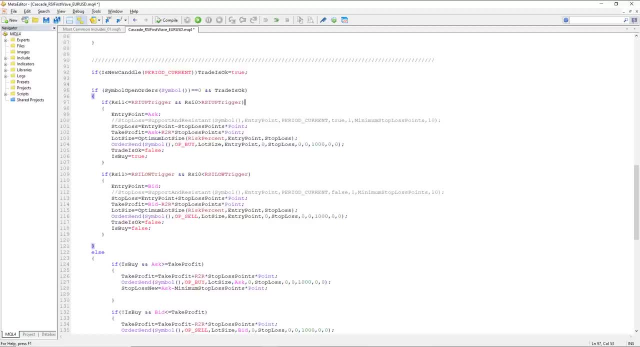 So this section of the video needs some knowledge about the programming with MQL4 language. If you don't have any experience, I leave you the link to the video. If you don't have any experience, I leave you the link to the video. 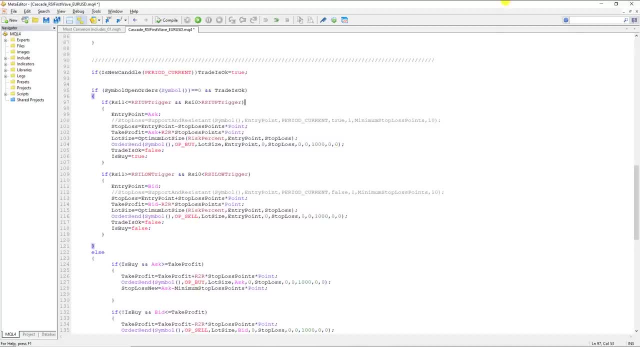 you that I taught it completely, from A to Z, and even it's suitable for those who doesn't have any experience in programming. I teach it. I taught it from very basics. So the first thing is that we have here is an if condition, and I check it whether it is the new candle or not. 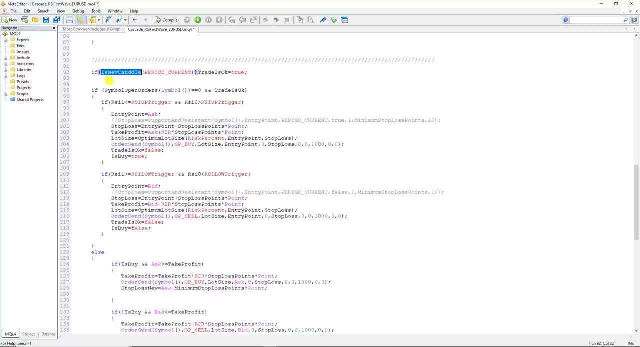 because I want to send a sell or buy order only at the beginning of the candle. We don't have such predefined function in MQL4 and I had to write it down by myself. I used three user defined function and at the end of this section I will explain how they are worked Once I wrote them. 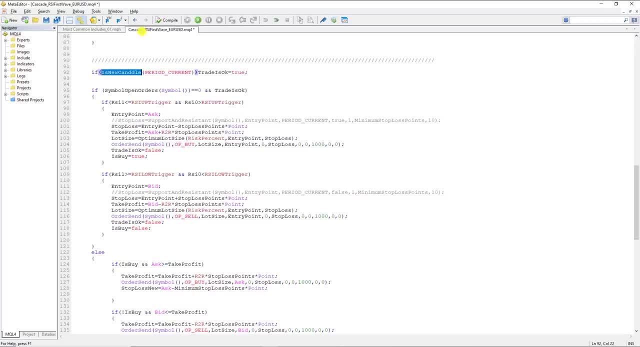 and now I saved them in my most common includes and for any new projects, even in the future, I don't have to write them down again and I just call them and use them. So if it's new candle, it means to buy order only at the beginning of the candle. So if it's new candle, it means to buy. it. So if it's new candle, it means to buy order only at the beginning of the candle. So if it's new candle, it means to buy it. So if it's new candle, it means to buy order only at the beginning of the candle. So if it's new candle, it means to buy. 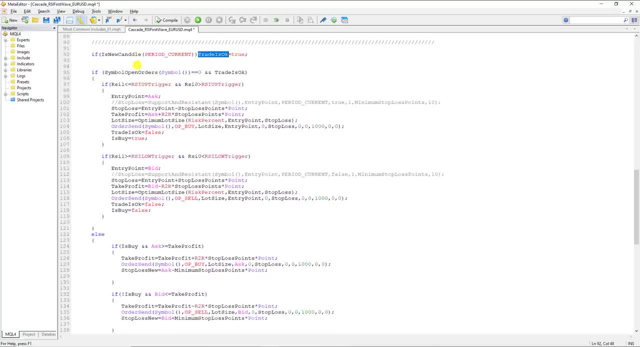 is OK, I am ready to send an order, So here I'll check. Here we have another if condition: I check the number of open orders for a specific symbol. If you are familiar with the MQL4 language, normally we use orders total to see the open orders. but this order totals return all open orders, But 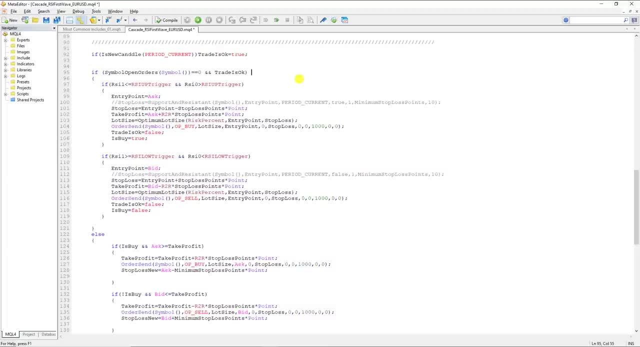 it doesn't separate them based on the symbols. for example, when we have 10 orders, orders totals return 10, but maybe I'm just interested in two of them which are related to the EURUSD. so I had to write down another user defined function which is symbol. 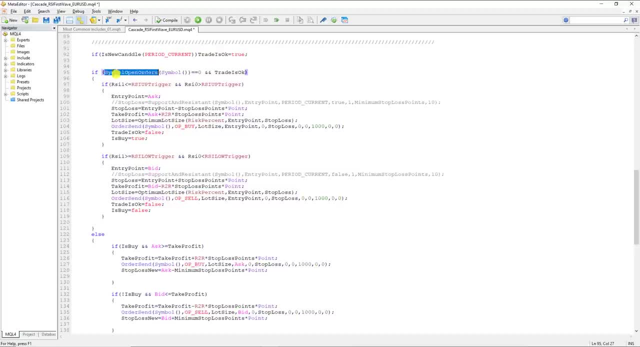 open orders, and I show you at the end of this section too. and if the open orders for specific symbols is 0, it means we can go for our open order strategy, not closing strategy. remember: these techniques, these cascade ordering techniques, is just for closing and optimizing our exit points, not for opening a new strategy. 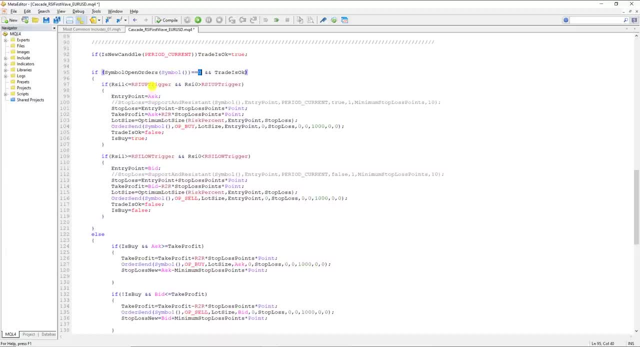 this strategy is very simple: it checks whether we are. it checks whether we are in the oversold RSI or overbought RSI levels. if, in contrast with what is common between people and new traders, I prefer, whenever I start to get into or enter the 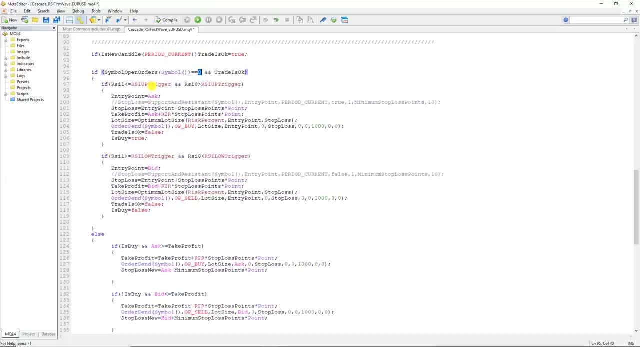 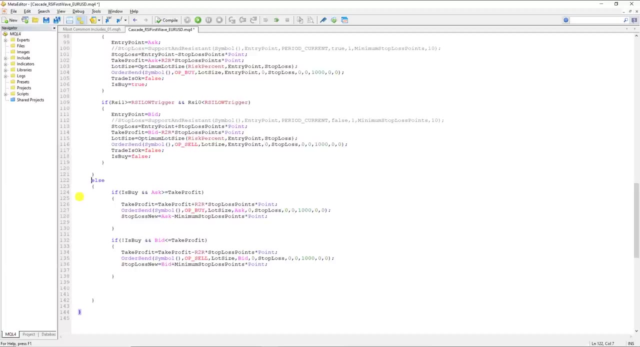 over sold area I wanna sell, and if I enter the overbought area I wanna buy. and this is what you look like, that and after that that process, after opening the first order from this else to the end, the process of opening second and third and fourth order starts. and here we have two separate sections. 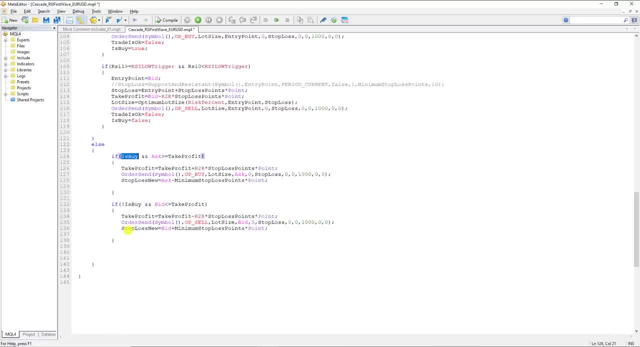 the first section is when the first open order is by and the second section is when the first open order is sell. it checks, it checks when, whether, when the ask is greater than take profit and the first order is buy, and then it update the take profit and update the stop loss and 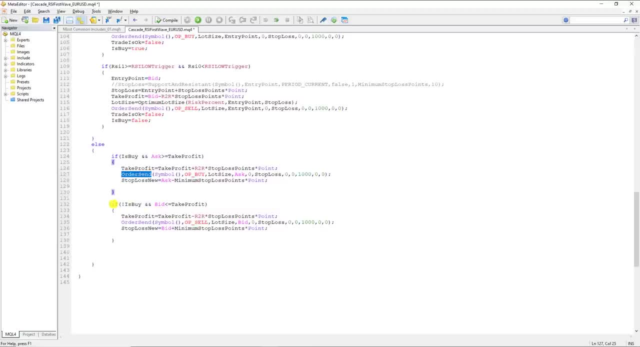 open a new buy order. but in this section, when the first open order is sell, the first open order is, so this one is means that it's not by the first order is not by and when, and at the same time the beat is less than take profit, it send. 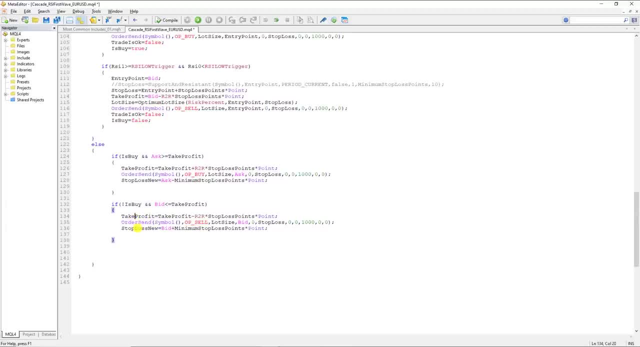 a new sell order and update, take profit and stop loss and after that for closing the orders. we should have another section here for closing the orders. when, for example, we open 10 orders and at the 10th order, uh, we goes back and hit the stop loss. 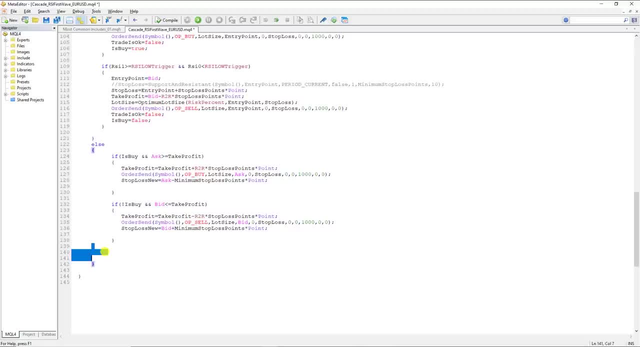 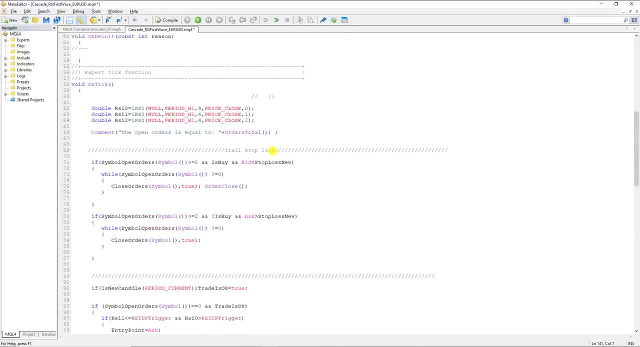 we should close all of them based on some technical issues. i prefer, instead of writing them, writing it down here, to write it down at the beginning of the code, which is trail stop loss, and closing it in this section. if, uh, if- the conditions met, then i sent the order of closing all open orders and again i use a user defined. 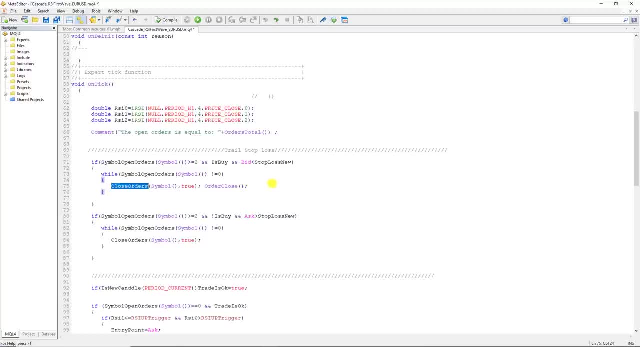 function, which is defined by myself. close orders: see mql4. language has a predefined function: names- uh order close, but this order clothes just close one order. i want to close all open orders only regarding a specific symbol. that's why i write: i wrote down this code by myself several years ago and i saved it in my most common includes. 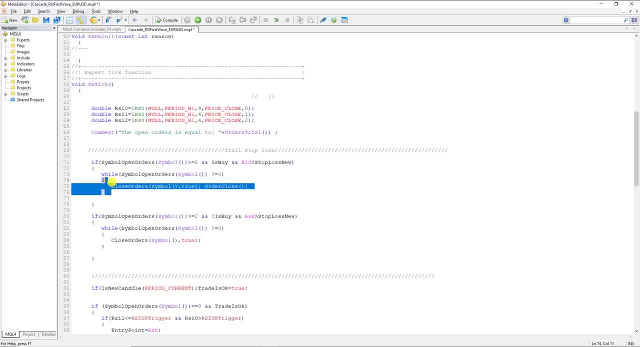 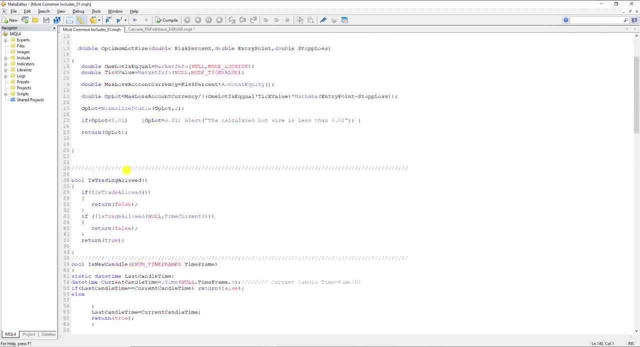 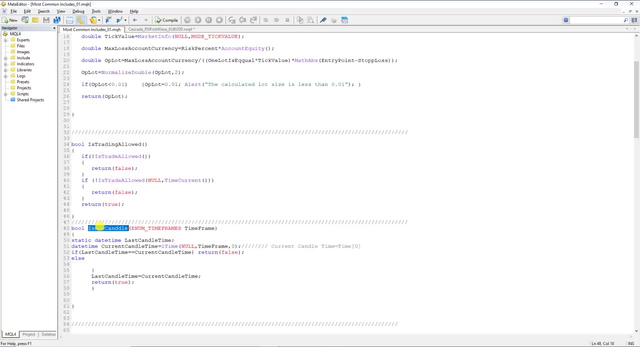 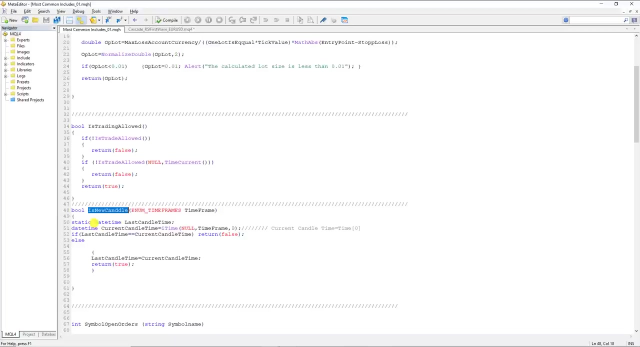 and when these conditions are true, then we those all open orders. and I mentioned three predefined, three user defined function which I'm using by myself. the first one, if you remember was, is new candle, because I want to send some. I want to run some part of the code only. 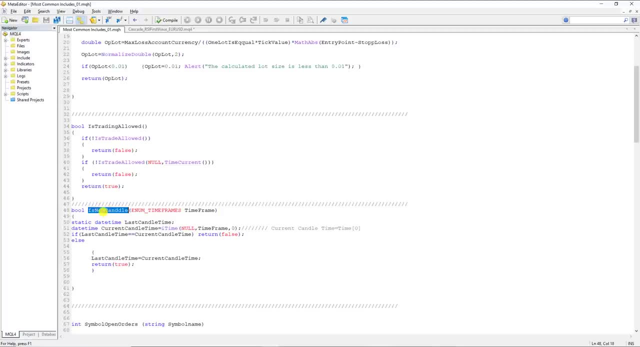 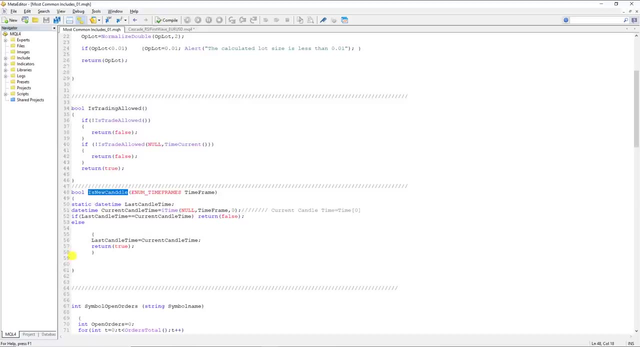 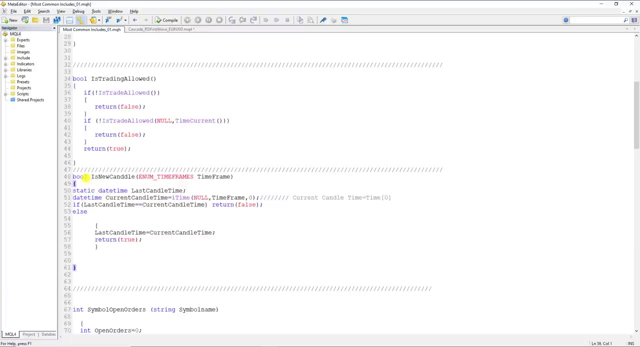 once per candle. so I had to define these codes, and I usually use it a lot in different codes. that's why I saved it. you can post the video and read it, because I think it would be interesting for you too, and if you are interested, I please leave me a comment to make a video for that. I will consider it for. 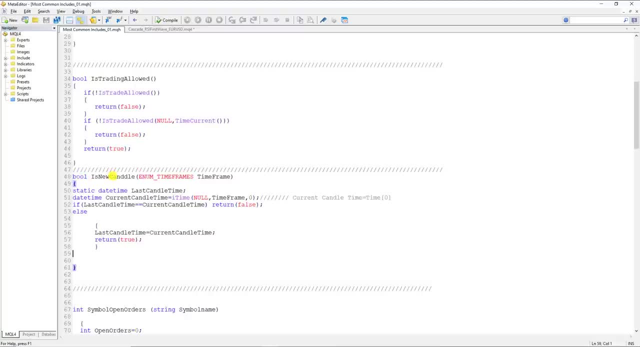 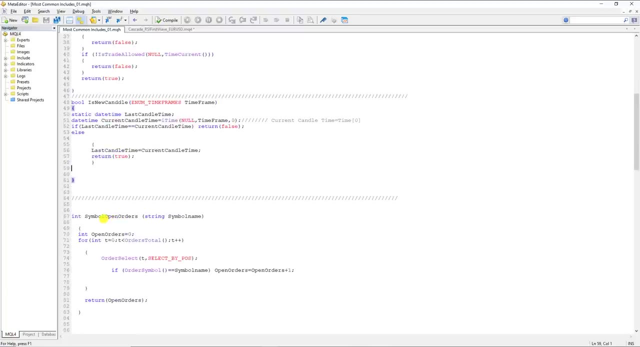 each of these user-defined functions. if you are interested in them, please let me know. I will consider them for upcoming videos. and the second user-defined function was symbol open orders, this one, which is again a predefined function, and this is why I saved it, because I want to send some. 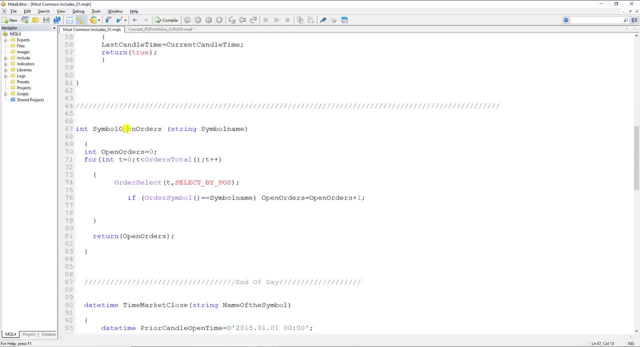 again, it's written by myself because I needed a lot in different projects and different codes. that's why I saved it and it just check the name of open orders with the symbol or name which is entered by a user and check it and if they were equal to each other, it we have a counter. 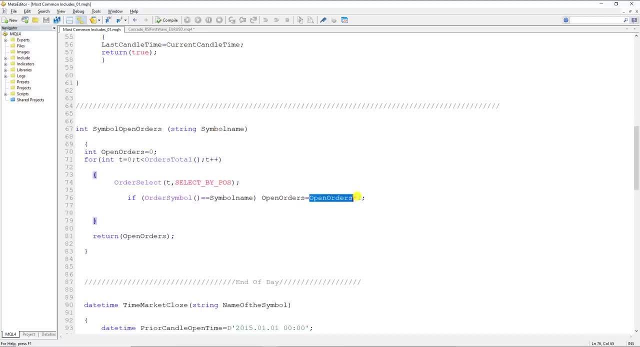 name open orders, open orders, and this counter would be added by one, would be increased by one, and it just count, count, count at the end. at the end it returns the number of open orders related to a specific symbol. you can again pause this part of the video too and read it more carefully, and if you want me, you please. 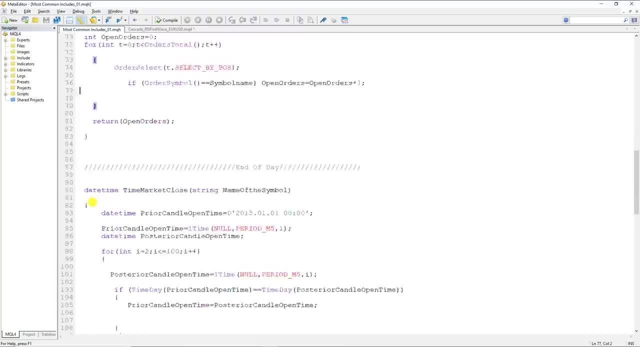 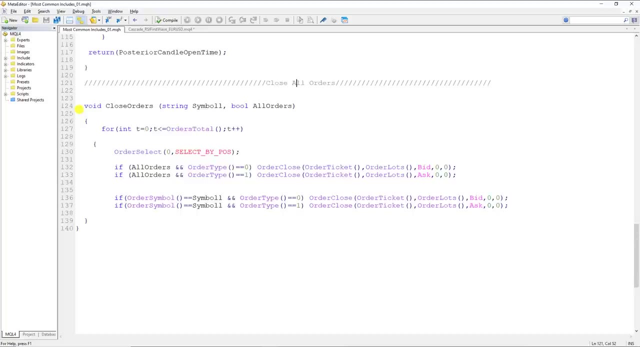 leave to have to make a video for the. please leave me a comment. and the last and not least but not least is the close all orders, which is written here. I suggest you to post this part of the video too, and look at it carefully. in the next section I will show you the performance and the. 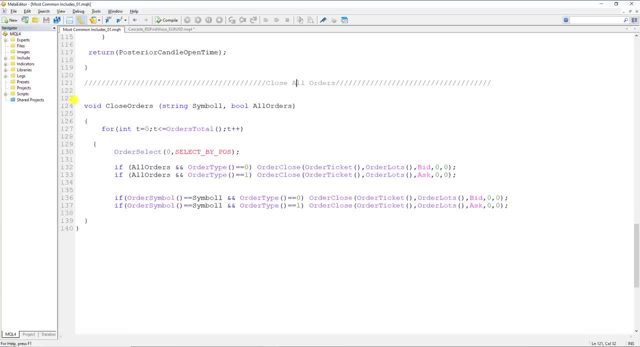 results of this strategy. again, I don't like to call it a strategy. I prefer to call it a technique to close the orders, because the it's just. it just make your strategy more efficient. first of all, you have to have a very good strategy to enter the market, and this strategy doesn't give you a 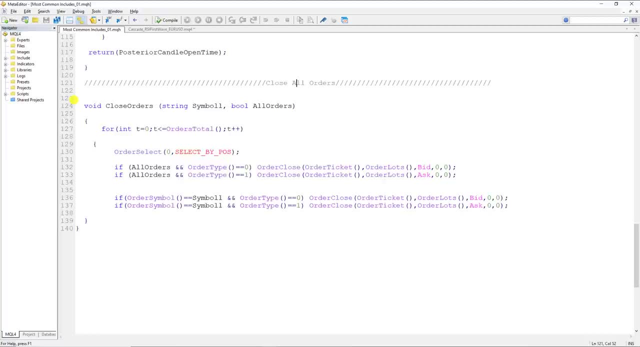 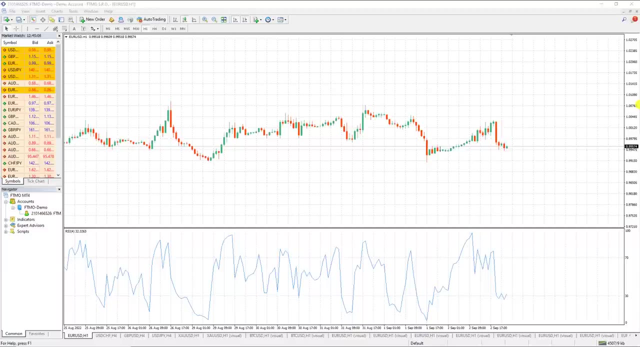 signal to enter the market. this strategy just help you to maximize, maximize your profit. in previous section I showed you how I program this strategy and in this section we use strategy tester to back test these techniques. first, the entry strategy is very simple: we just enter this: enter the market by, based on the RSI and whenever. 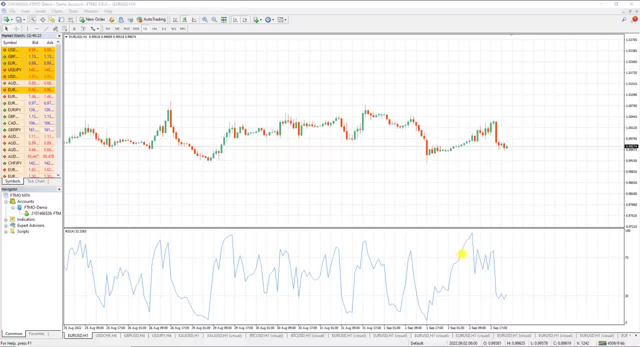 rsi is going, for example, into the overbought area, we send an order. we hope that the it continues the trend and whenever it goes to oversold area, we send a sell order to and hope that the trend will continue now and then, after opening the first order, we check it whenever we hit the take. 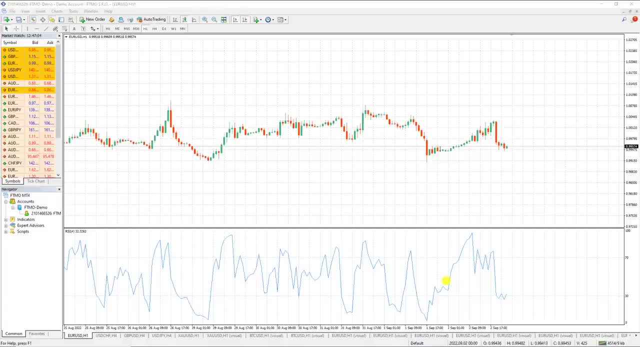 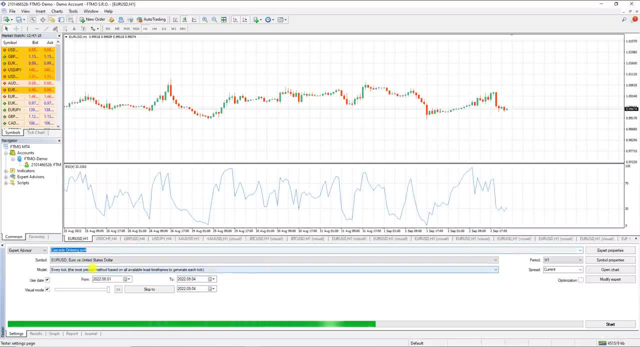 profit. uh, instead of closing the order, we open new orders, and we do that as many time as possible until we hit stop loss. so first i, from here, i opened a strategy tester. the strategy tester is opened. i chose the cascade ordering code, which is the code of this strategy, and from here, i choose euro, ust. 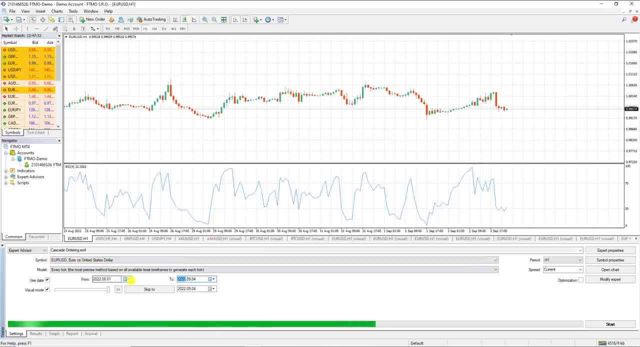 and i, from here Here, I use the date from when to when I want to test this strategy, from 1st of August to 4th of September, And from the expert properties in the testing, I want my initial value be 100,000 USD. 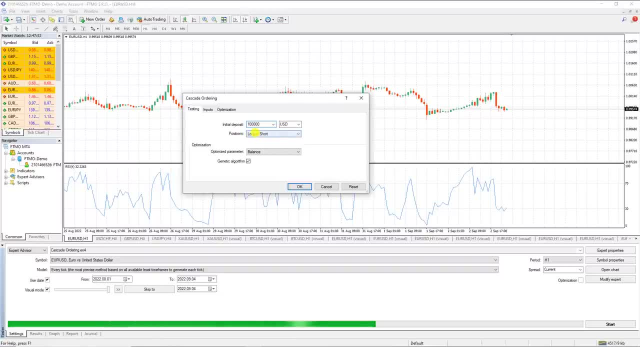 I want it to be able to open, buy and sell or long or short positions And the inputs of the strategy, the inputs of this code is written here and we can give them initial values. If you are not familiar with it, I again leave you the link for its course and you can find it and see the course and learn how to use it. 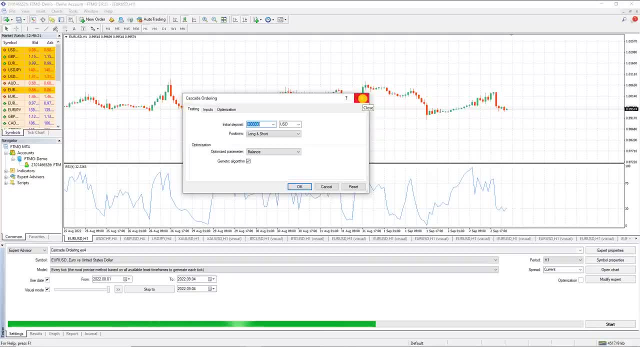 So now the strategy tester is ready and I press OK. And now the period. I want this strategy, this code, be run on the one hour time frame and the speed would be controlled from here. Everything is controlled Now. if I press the start, the strategy would start to run. 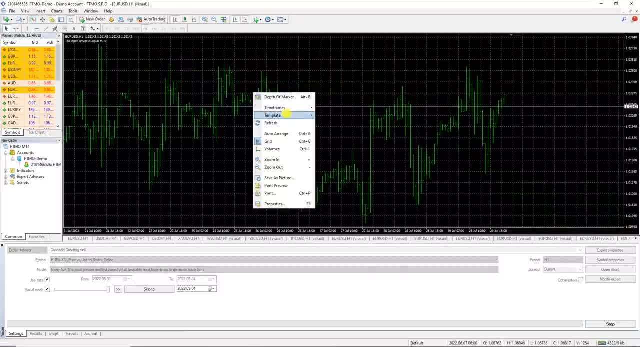 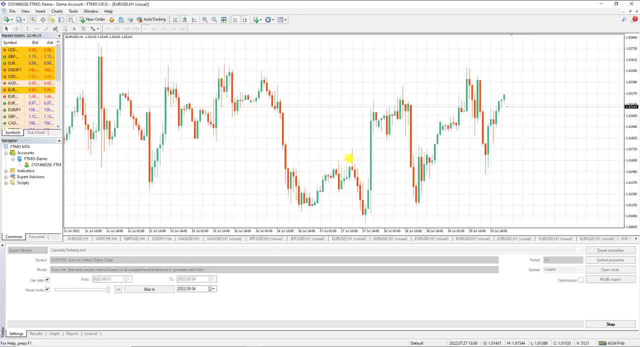 I press start and I add a template, a clean one, which is used here, And We it starts to running after downloading the data of previous months for these euro USD Symbol. it takes a while, it's downloading And we wait for it, and it's already download and I press run and it's still running. 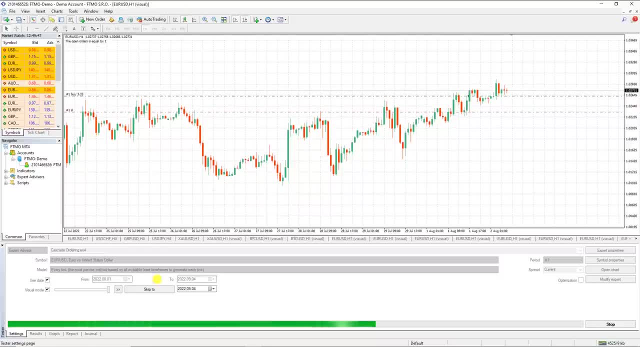 See, the first order is opened and it waits to go higher And if it goes back and hit the stop loss it's over. We lost it because Our entry was not correct. but if it's go continue and go in our favor, then it open new order. 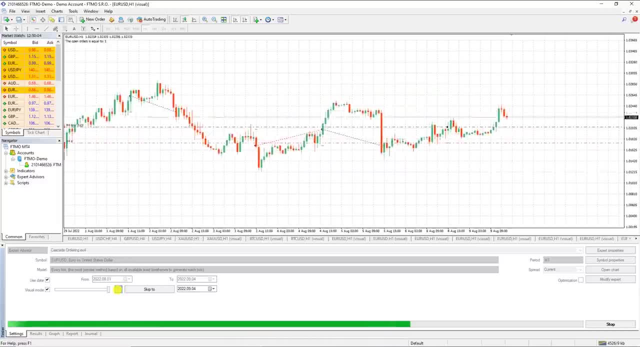 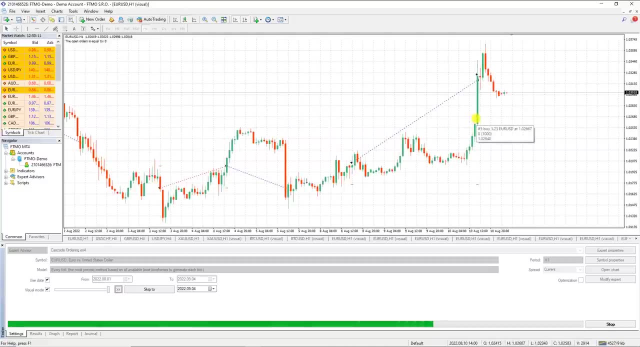 In this case it didn't go in that way. We wait with, and now here it goes, in our favor. it opens the second order and the third order was opened here and it goes higher, but it couldn't reach the point to open the force order and it goes back and here it close. 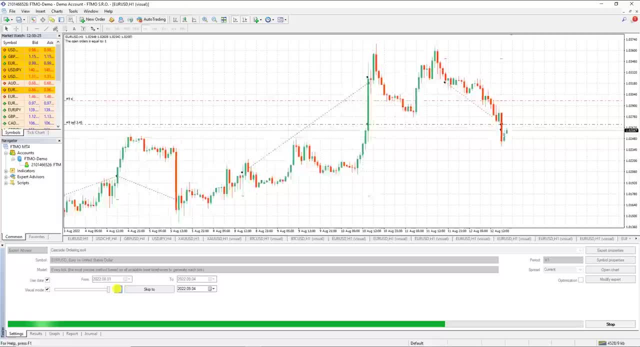 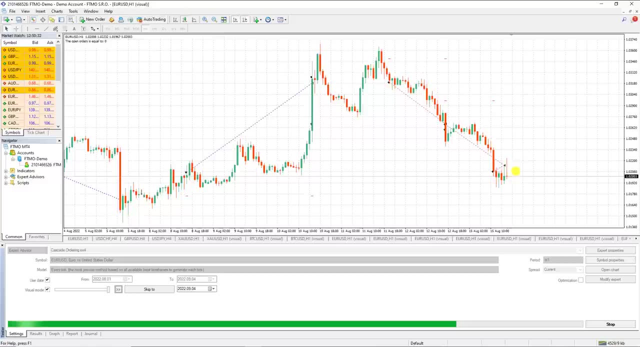 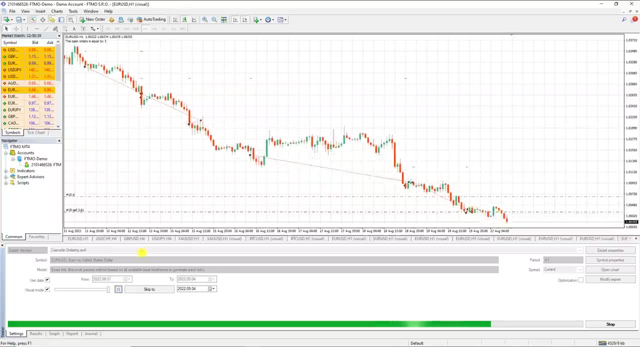 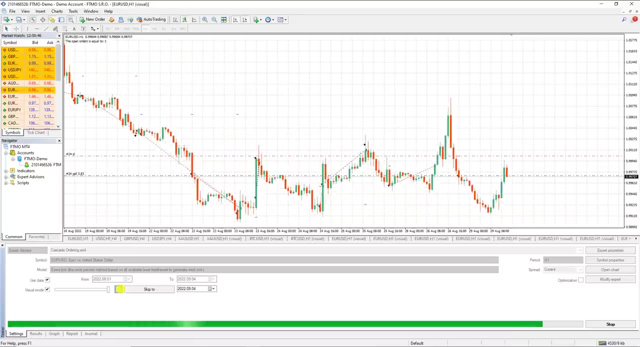 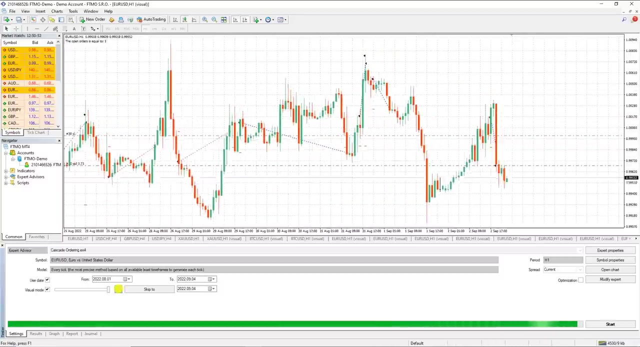 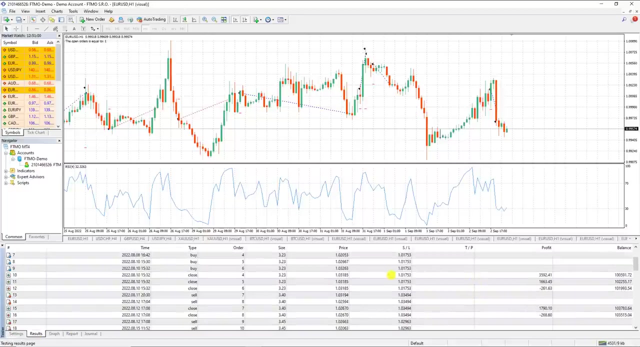 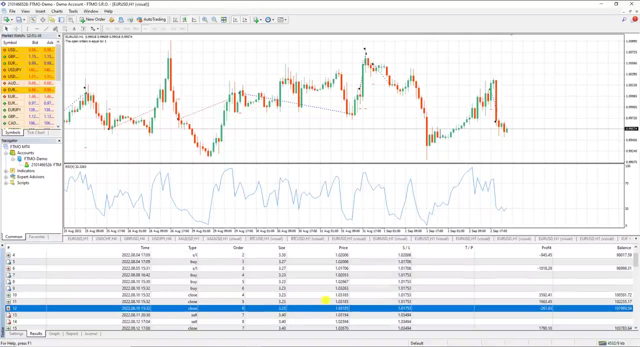 Or Orders. Now again, Again, I comes down. The first order was opened and the second order was opened by it couldn't reach the third order, And It continue, As we can see, It's going very fast. But I think, if we see the results we can see here, for example, here, as you can see, for example, here, as you can see, we have three orders. it couldn't reach the force orders. 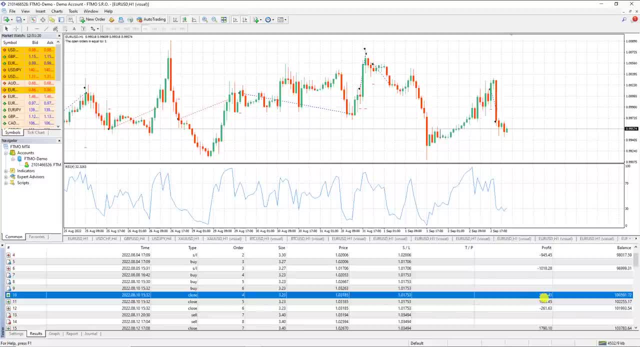 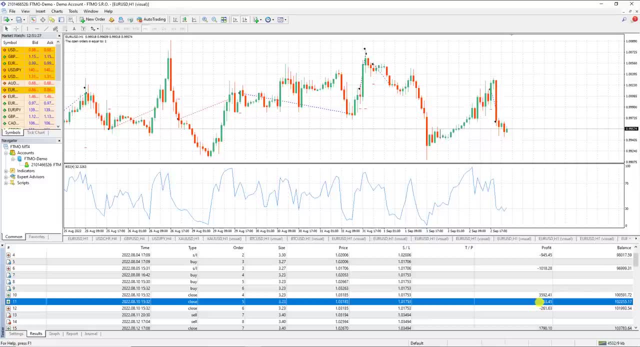 The first orders closed with a $3,592 in profit. One on the second one is one hundred, It's One thousand six hundred sixty three dollar, and the fourth, fourth, third, third, one minus two hundred sixty one dollar is lost. 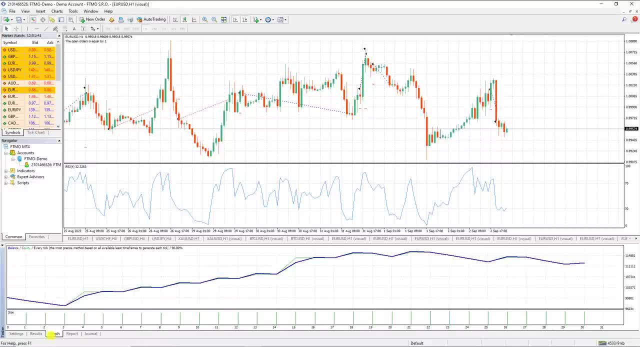 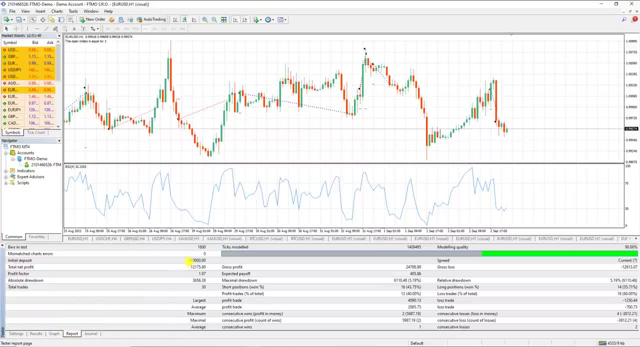 And if I goes down, we can see all the results. The graph is like that. It's going in this, The sleep page, very beautiful one, And now, as you can see, this is the result of this strategy. Oh, 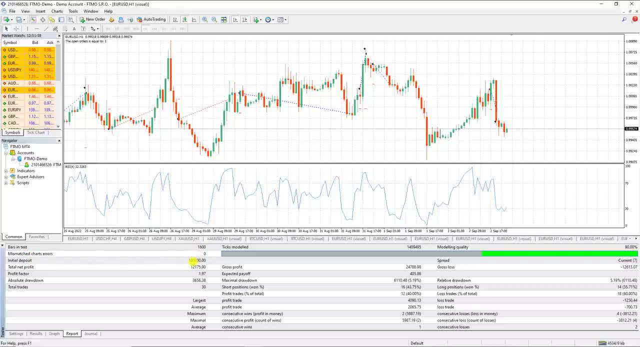 The initial deposit was One thousand one hundred thousand dollar. We gained twelve thousand dollar. twelve thousand twelve thousand one hundred seventy five dollars and absolute drawback is written here: The total trades: 30 trades were open in this one month. The short positions that we won is forty three percent of them closed by profit. 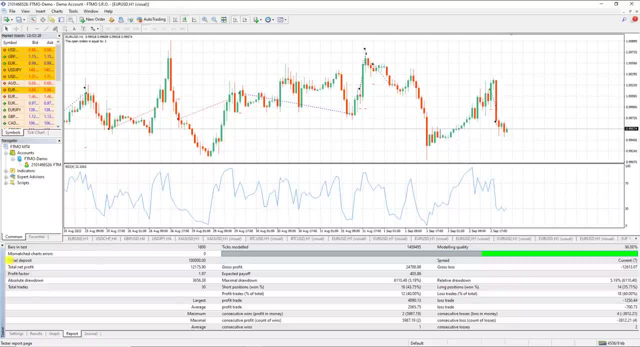 And you can see all other data. It was related to this strategy but at the end, without risking whole balance, with having only risking one percent of our balance, because whenever we open, we open an order- the stop loss was in a place which, when we hit it, we only would have lost one percent of our balance. 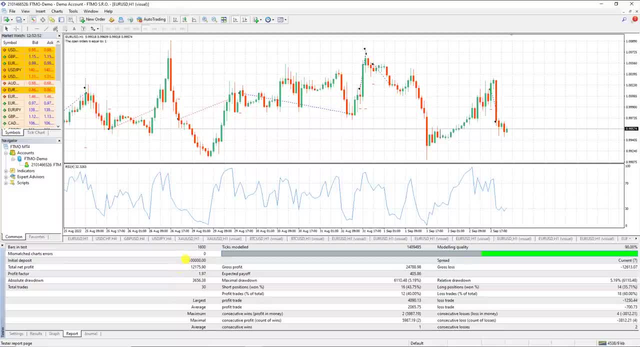 So we all, with only with having a logical stop loss, We gained About twelve percent of our balance in one month. Before finishing this video, I want to notice that all the lots and points which were used and mentioned in this video, actually they are for just educational purposes. 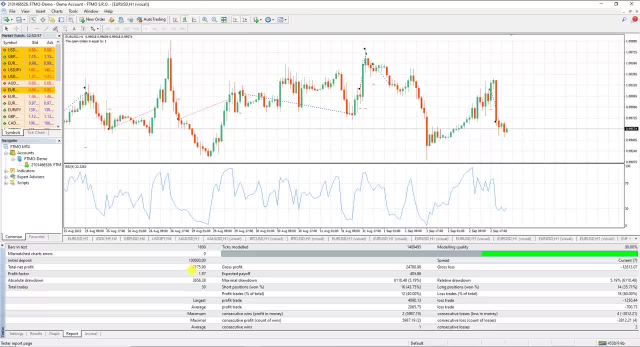 For example, these one lots that I mentioned is should not be always one lot. It should be based on the logic and risk to reward and what is optimized, optimized lot size for your tradings. It should be calculated. But here I just wanted to see to show you. 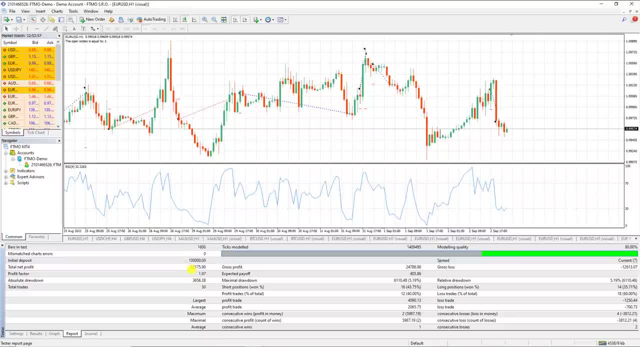 The mathematics and I wanted it to be as easy as possible. That's why I used one point, one lots, ten points for stop loss and twenty points for take profits. It can be anything and any combination, and you can do it even more efficient than me. 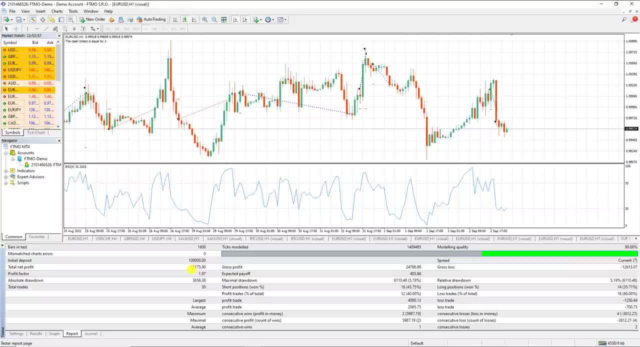 And the second one is: I want you, I want to mention you again that the interest strategy is very important. This strategy, or it's better to say techniques that I showed you in this video is actually just a strategy. It's better to say: techniques that I showed you in this video is actually just a strategy. 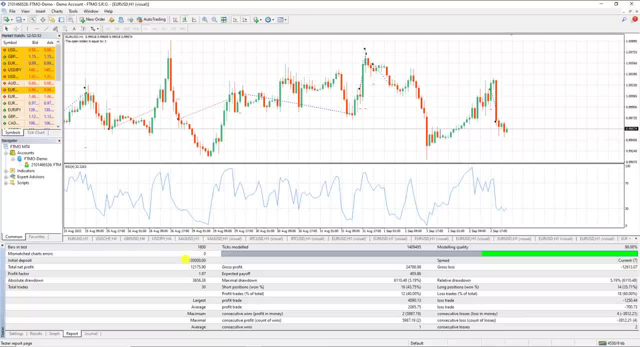 It's better to say techniques. that I showed you in this video is actually just a strategy And techniques to gain more money, to be more efficient and to increase and multiply your profit. It's not an entry point strategy If your interest strategy for enter the market is not a good one and it's not a profitable one. 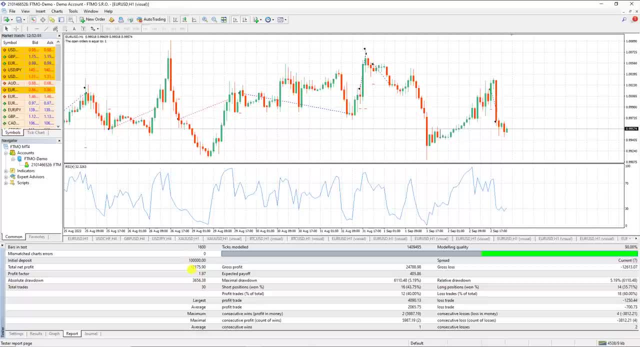 This techniques does not help you a lot. I hope you enjoyed this video. If you enjoyed it, please hit the like button. So the algorithm YouTube will introduce us to those who are interested in this subject. So the algorithm YouTube will introduce us to those who are interested in this subject.